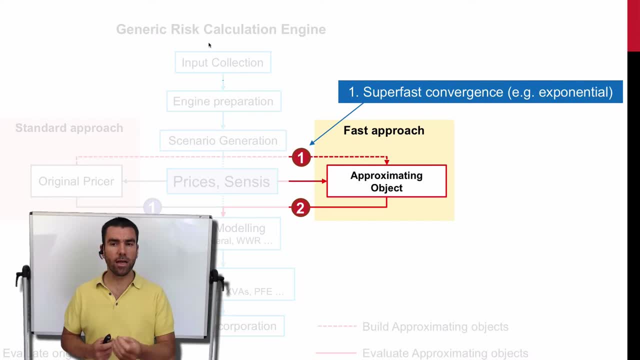 First of all, step number one is to be super fast, convergent. That is that we need to be able to create an approximating object that is a very good replica of the original pricer, so that the error is very small, but calling the original pricer very few times. 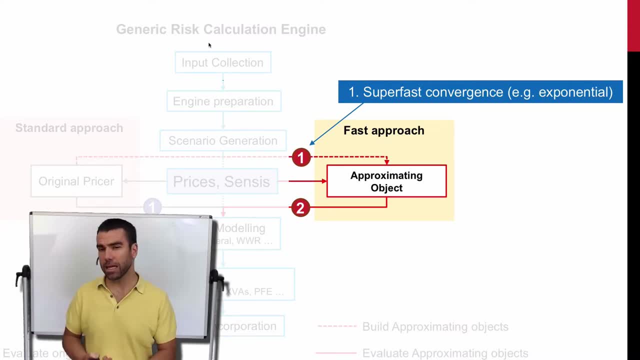 Otherwise the exercise doesn't make sense. So it needs to be a technique that from the mathematical point of view, converges to the original function, to the original pricer very fast, For example, ideally exponential. You know, in practice and reality we cannot hope for better than exponential. 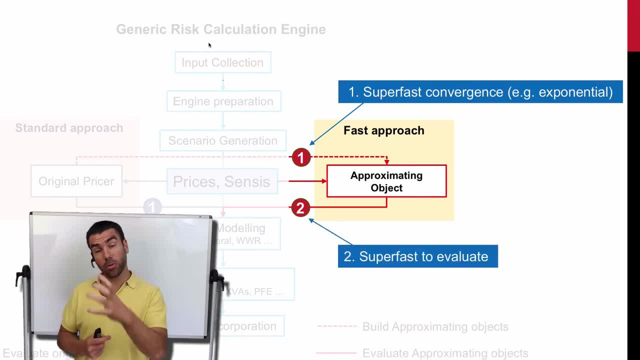 Now the second one is it needs to be. the object that we create has to be super fast to evaluate. Why? Because otherwise it defeats the purpose of the exercise. Third, it needs to be very stable. We are going to see in future videos, in fact, that sometimes you can have things that seem to be. 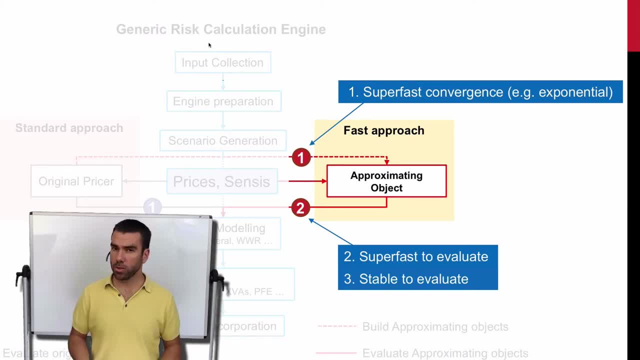 fast and easy to evaluate, but then, when you implement it in a computer, you can have numerical instability. So we need to make sure that we don't have any of those. Now, as a fourth one, as a fourth property that we wanted to have is that we need to have a good control on the error. 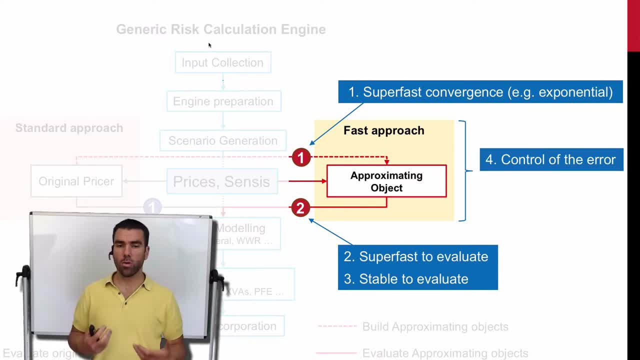 This is quite important because, in implementation, we want to make sure that, before the whole calculation finishes, we want to make sure that we have a good control on the error. So we want to make sure that we have a good control on the error. So we want to make sure that we have a good control on the error. 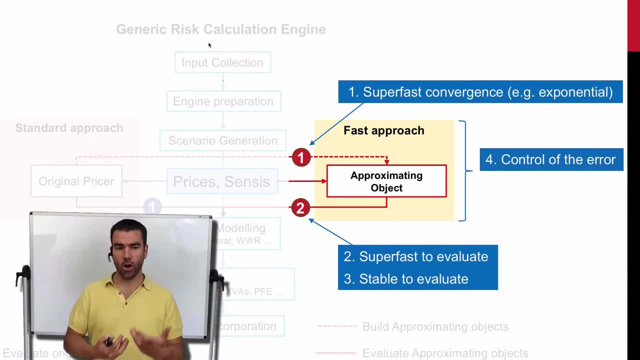 know what error we're going to get. So we're going to have a sense of the approximation that we're using And on that way we can calibrate it on step one accordingly, Or even, in the worst case scenario, we can reroute the calculation through other alternative routes that we can create in the code. 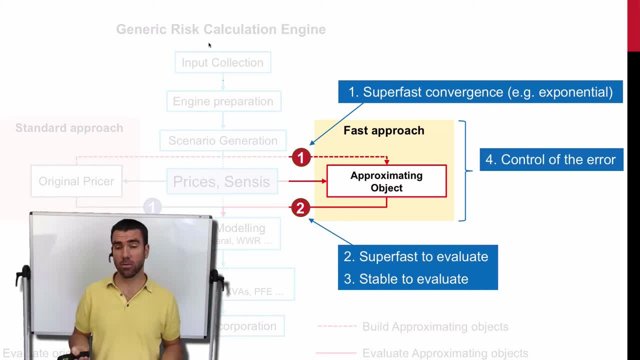 to make sure that we get to a reasonable result. But we want to see this before we get to the end of the calculation, So we want to have some control of the error, And so we just want to make sure we get to a reasonable result. So we want to make sure we get to a reasonable result. 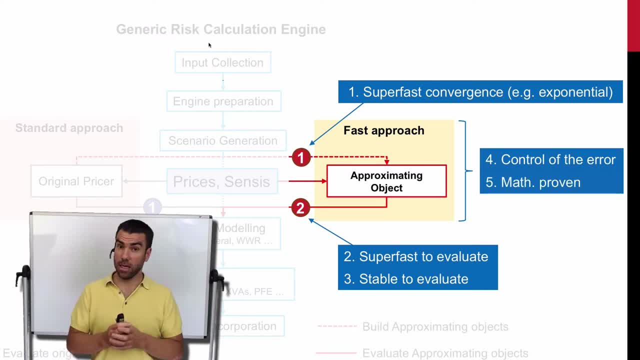 So we want to make sure that we get to a reasonable result. But we want to make sure we get to a reasonable result. And a fifth, something that is a very, very awesome important in practice is that the whole framework has to be- or ideally, 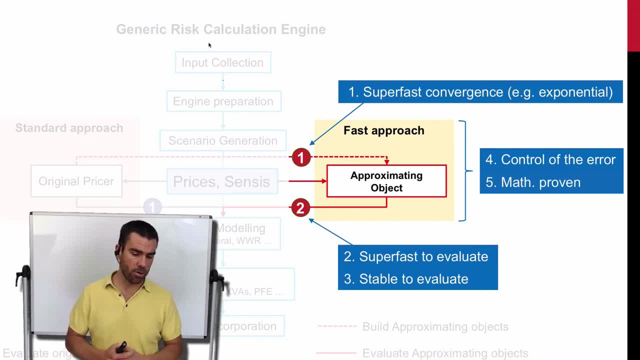 you want it to be mathematically proven. In fact, I've spoken to a number of mono-validational regulators about this type of approaches And when they see that the solution it is mathematically solid and robust, they feel much more comfortable. 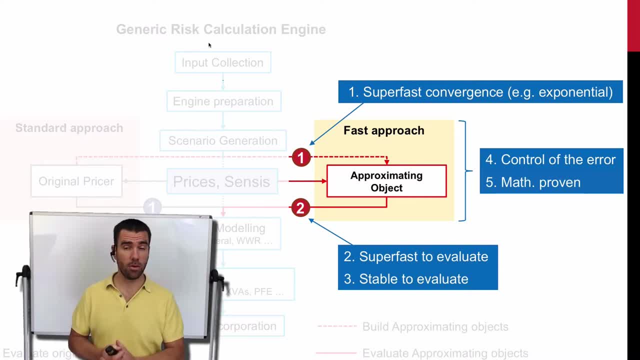 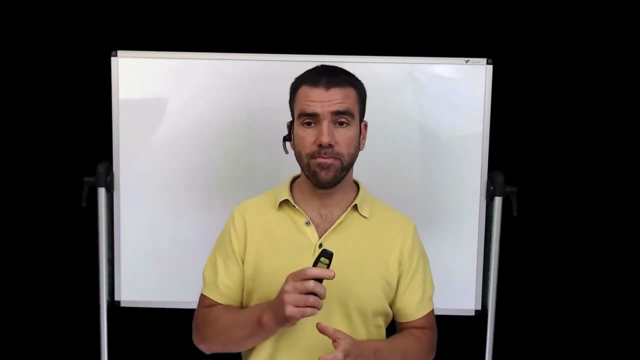 So it is something that that is also quite, quite a must, something quite important that we want to have now in this session. we are going to focus especially in step number one: super fast convergence. that is going to set the ground for anything else afterwards. so let's focus in, in, in that. now let's talk about different. 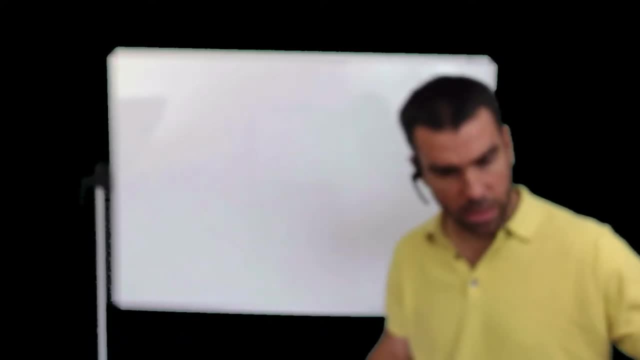 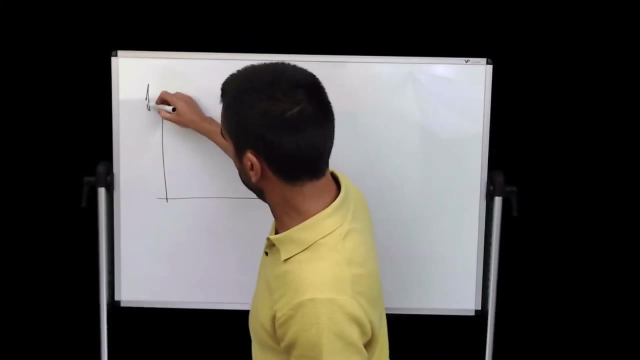 approximation formulas that we can have. so let's suppose- let me get this here- let's suppose- that we have a function- x, f, okay, something like that- and we want to approximate this between two points, a and b, okay, okay, what is the? what is the first thing that we can do? well, the obvious thing is: 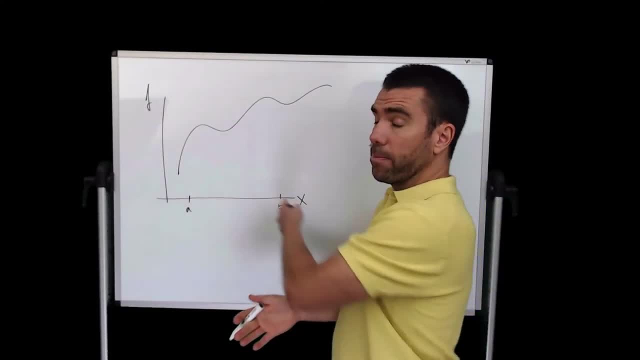 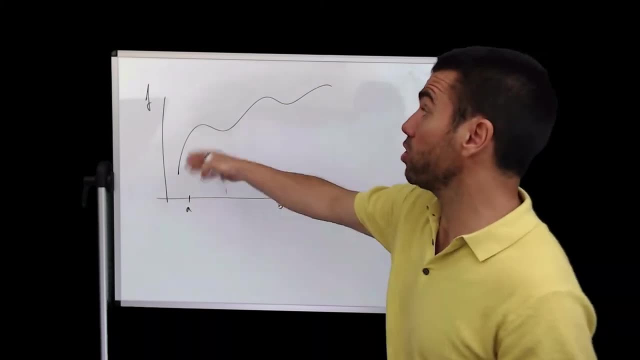 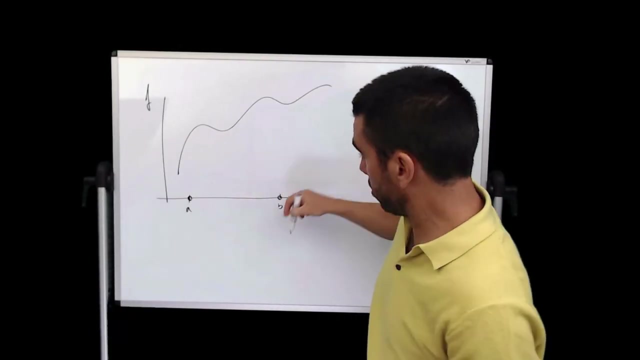 we- and let's suppose that we want to use, to make the plot easy, four points, right. so we have to distribute the four points here and we know nothing in principle about the function. we don't know what this black line is. so what do we do? we know nothing about the function. we pick equidistant points, so obviously the two. 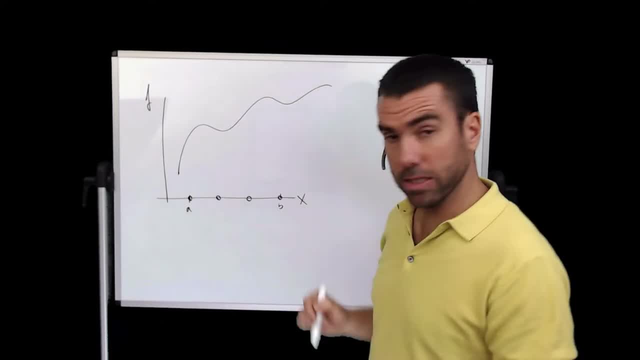 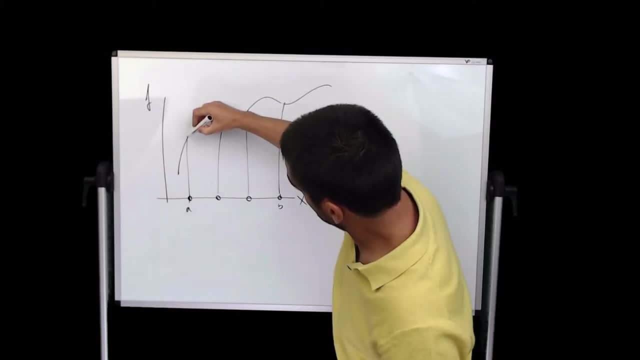 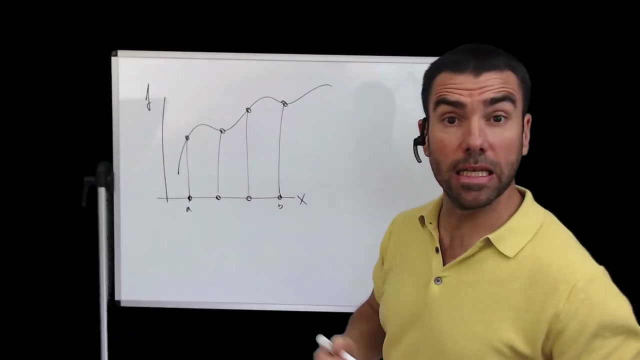 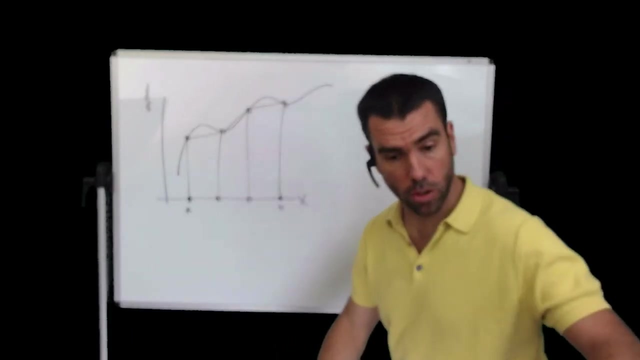 extremes and then two points here so that they are equidistant right, and then we call the function in these points here we obtain these values, and then, when we have these values, we can think of doing, for example, some linear interpolation right, or we can think of doing some sort of 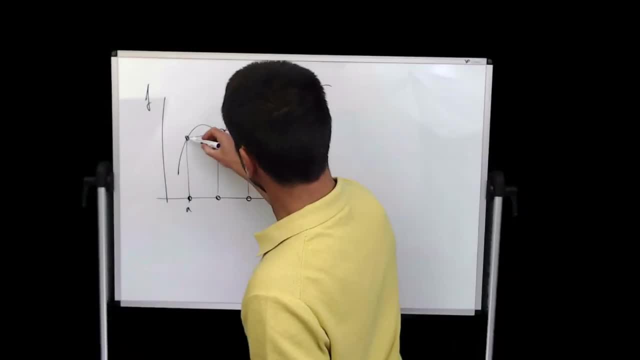 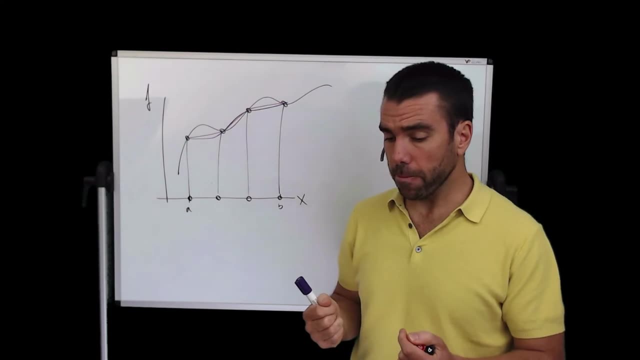 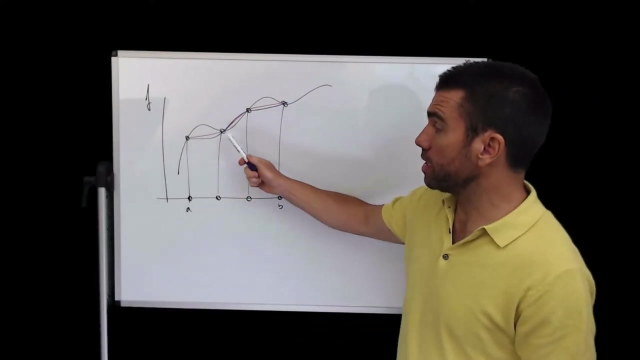 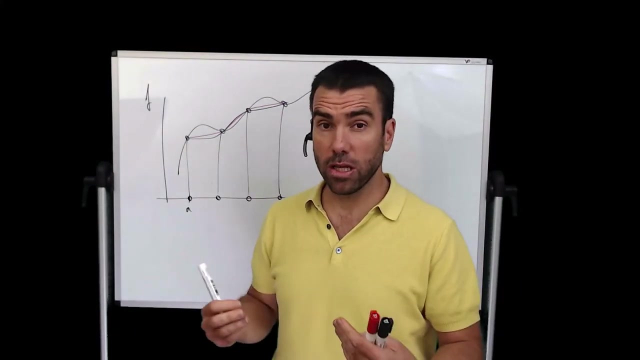 of spline interpolation. it's quite popular as well. something like this: all right. also something that we can think about is it is it is doing a treating a polynomial, because we know that when we have, in this case, four points, there is one unique polynomial of degree three that goes through those four points and in general, when we have n plus one points, 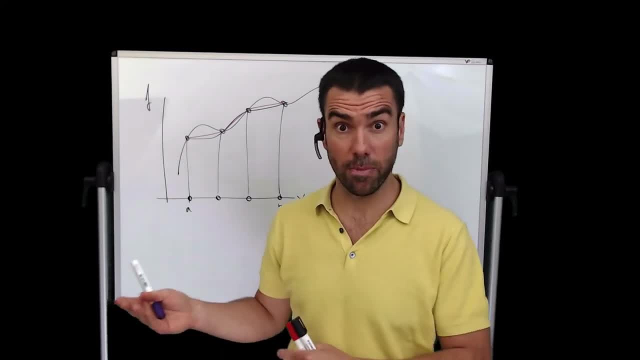 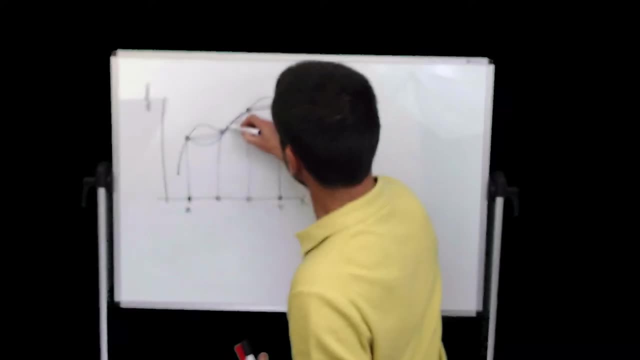 there is a unique polynomial of degree n that goes through those points, and then we can think of n plus n plus one points, so we can get- uh, we can basically calculate it as well- which is going to be something different to the other two. all right, so that's another approach. another approach would: 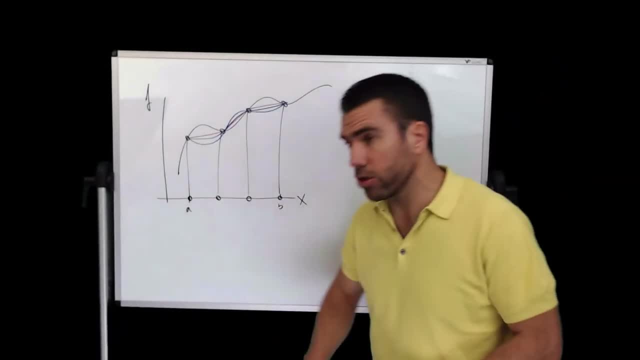 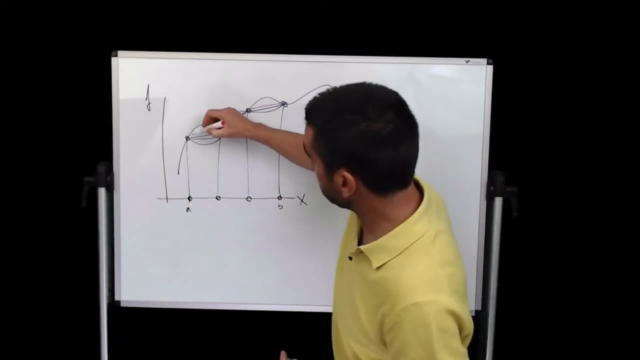 be, for example, the popular regressions in the regression techniques. what we're going to do is we're going to regress cash flows from the future for the derivative, from the different scenarios of the risk engine, and then we're going to get like a cloud of of points of possible cash flows. 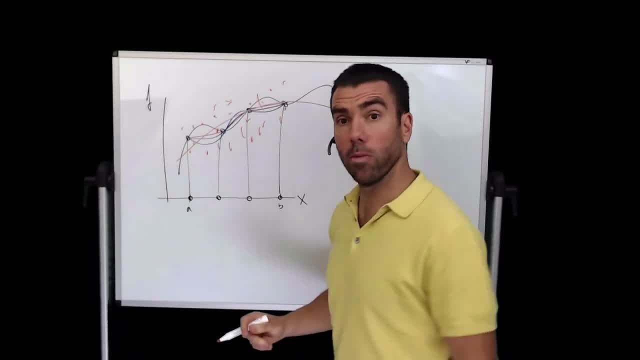 and here we're going to do a regression of the risk engine, and then we're going to get like a cloud of points of possible cash flows. and here we're going to do is we're going to fit a polynomial or a number of polynomials to it right now, and then 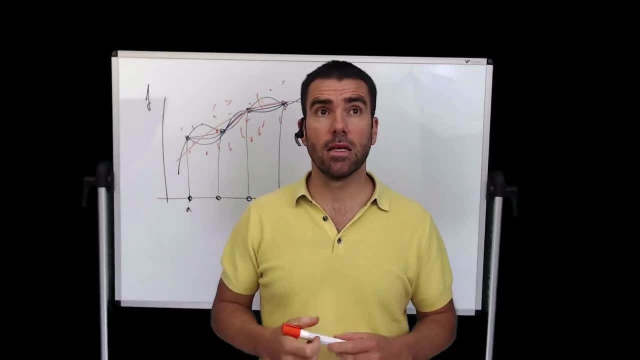 another approach that they that can be used is something like a machine learning type of type of techniques that are starting to to be out there. in fact, i had a talk, very interesting talk, last year about it. having said that, it is very interesting, but so far the results are there. 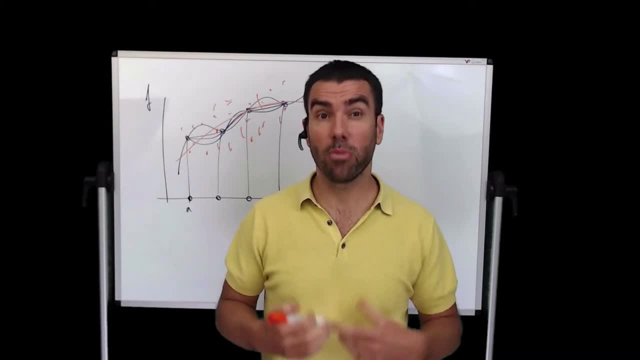 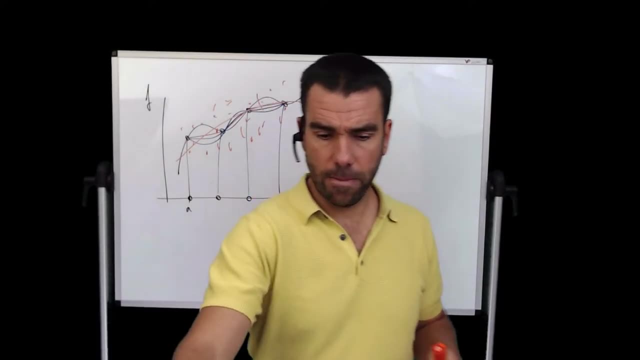 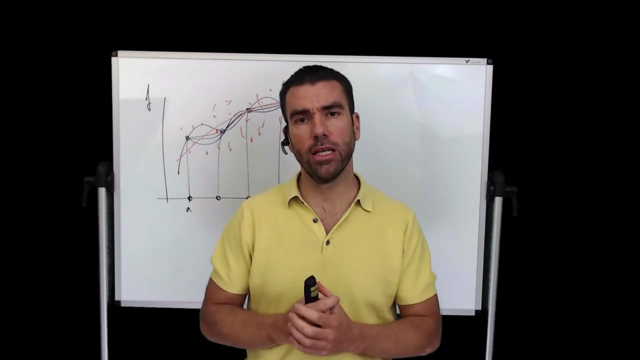 is nothing. personally, i haven't seen anything convincing from the practical point of view anyway. so we have this type of approaches. so let's, let's see now. yeah, let's see now. we're going to introduce now the chebyshev framework into into this like another approach and we're gonna see. 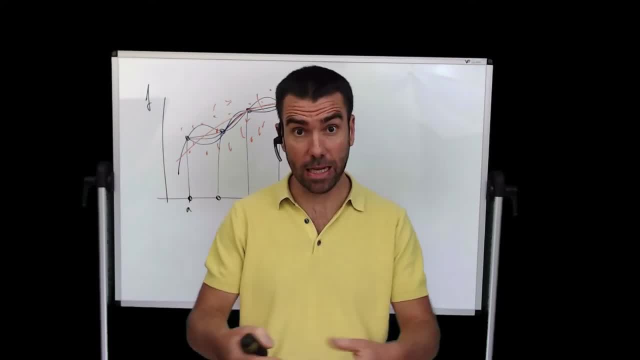 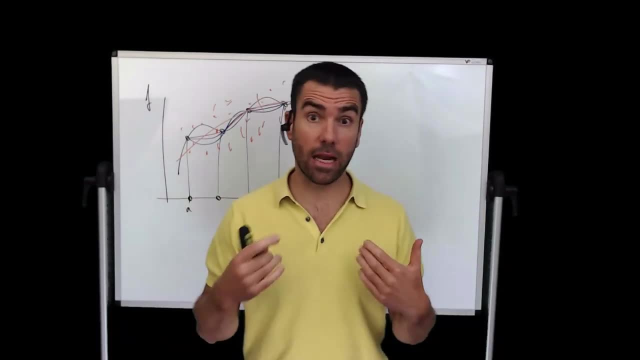 how really, and we're going to demonstrate to you mathematically and and in a very solid way, how the chebyshev framework is better than any other thing that we can think of, at least that that i know of, and and i think that exists in the in the industry. now, everything that i'm going to 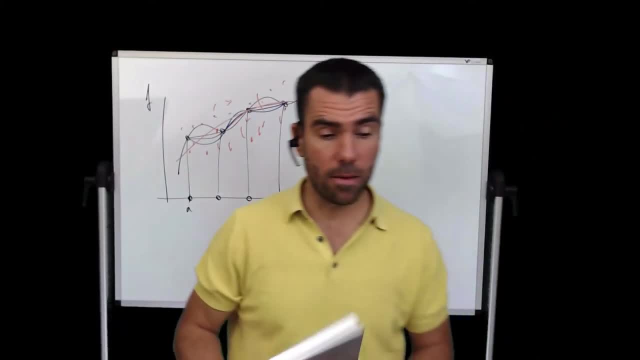 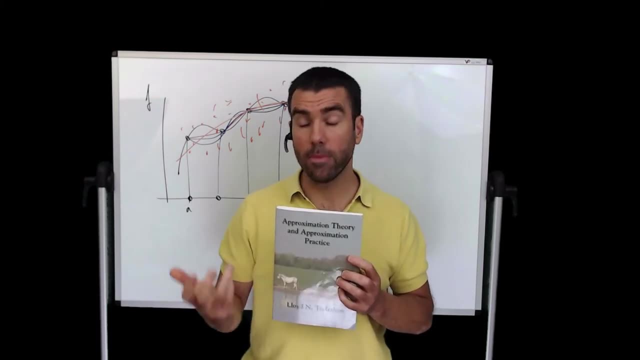 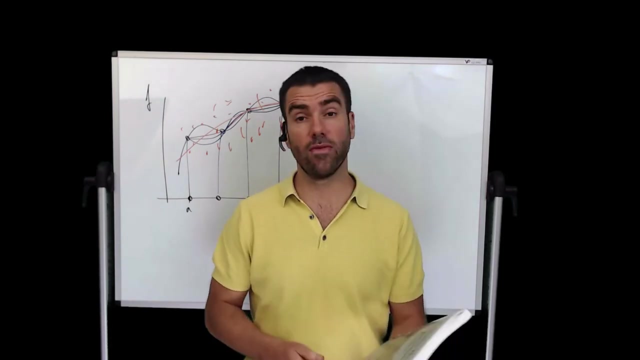 say or what, not everything. most of the things that i'm going to say are based on this book. if you want to get deep into this, into this, into this problem or approximation theory, i strongly recommend this book: approximation theory and approximation practice by professor trefessen. 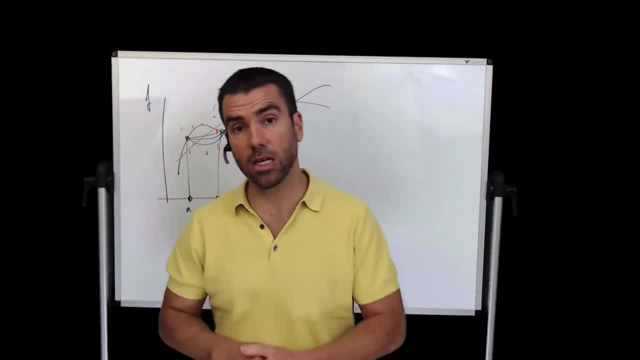 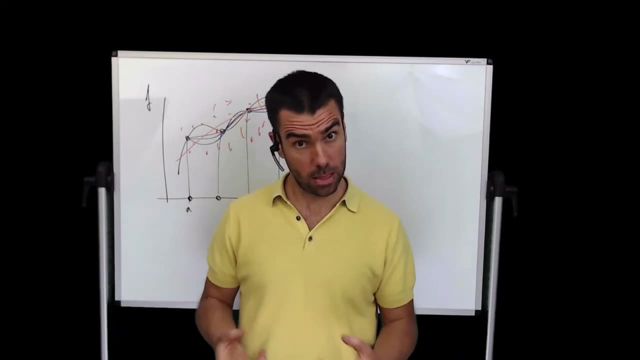 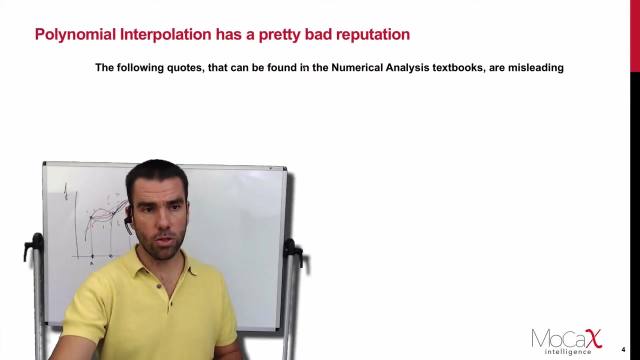 from oxford university. i met him a couple of years ago. he's a super nice guy and and i strongly recommend that if you really want to get into into this subject, let's start with that book. it's an amazing book, it's really really good. so let's go now into into. 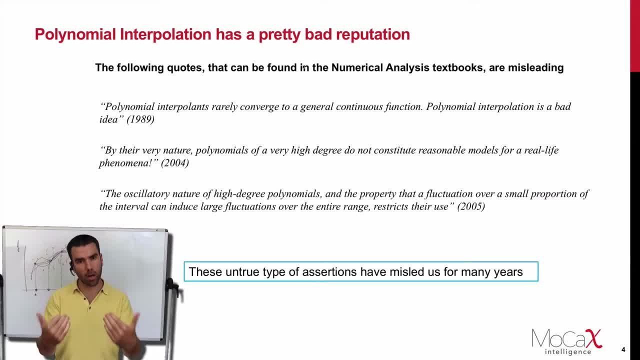 the let's, let's, let's transition into the problem, that we want to tackle it with more detail and then the the solution that we, that we are going to suggest, that we're going to discuss polynomial interpolation. polynomial interpolations have a pretty bad reputation. now you can find the literature, the following: 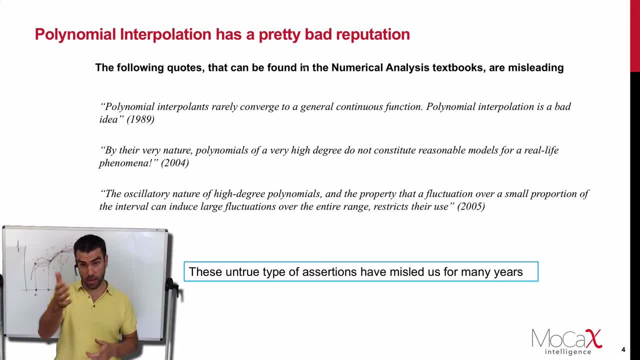 sentences that you can see in the screen. in fact, i've taken this, this, these phrases from trefesson's book, for example. you can find that polynomial interpolant really converts to a general continuous function. polynomial interpolation is a bad idea. also, in the very nature, polynomials of a very high degree do not constitute reasonable models for a real life. 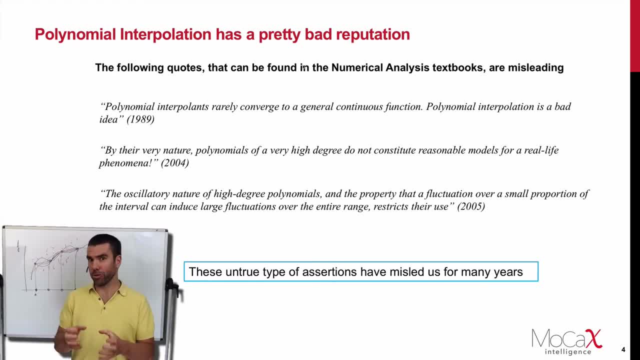 phenomena. now, this type of things are as well- as i'm going to do a little bit of a demonstrate to you in this session- are untrue and have misled us for for many years, in fact, when we were studying university. there's been a. it's basically most of us has been misled by this type. 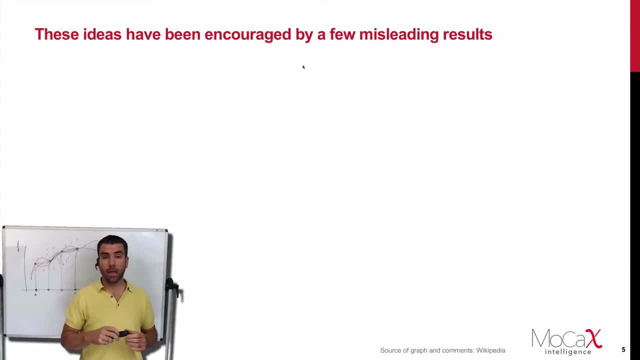 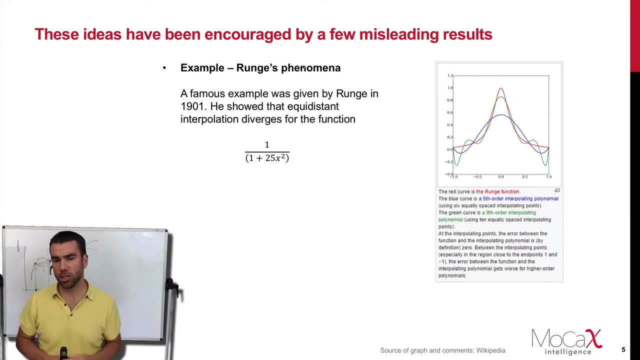 of things. so now, these ideas, in fact, have been encouraged by the following results: if we think- let's think of the runke function which you can see in the screen- this runke function- it is a super smooth- is analytical, I mean, it cannot be smoother and, in spite of that, the approximate. 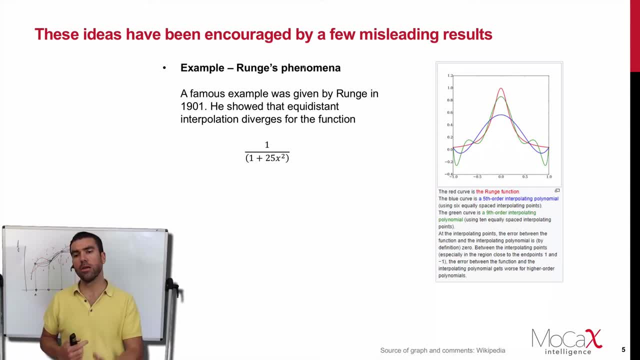 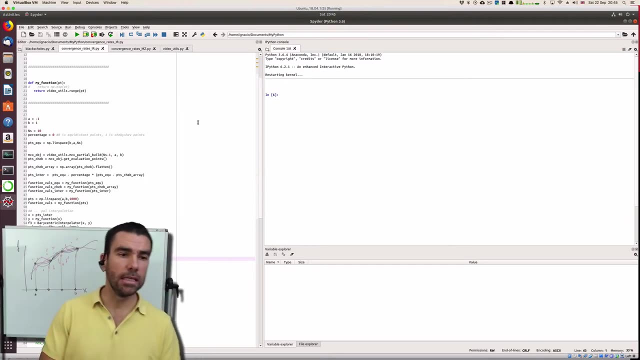 if you try to approximate this runke function with a gridded point, with a polynomial, it diverges. let's have a look at this. I have here a little code. let's go to my linux environment, in which I have a, in which I have a little script that I've written in python and, for example, let's start: 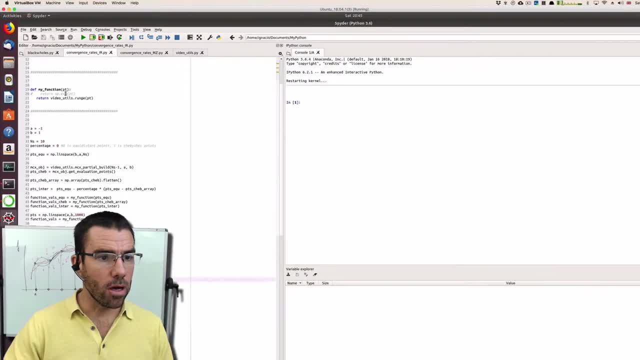 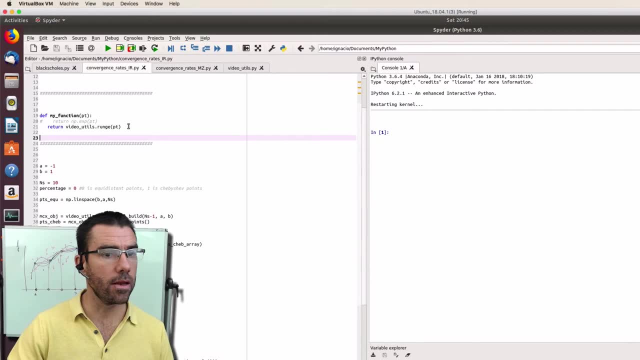 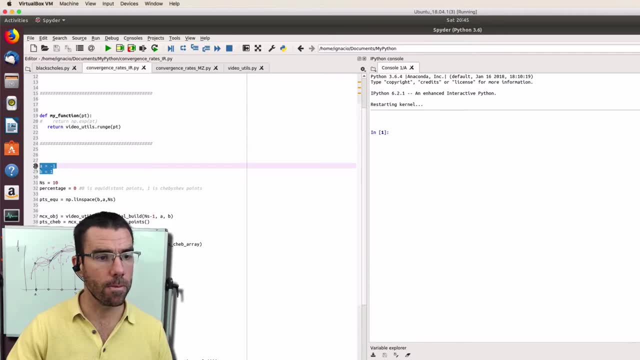 try to interpolate it between the points minus one and one, right, And let's start with 10 points, okay? So let's run this, And what you can see in the screen now is two graphs. One of them, the green graph that you can see here, is the actual function, and the blue one is the polynomial. 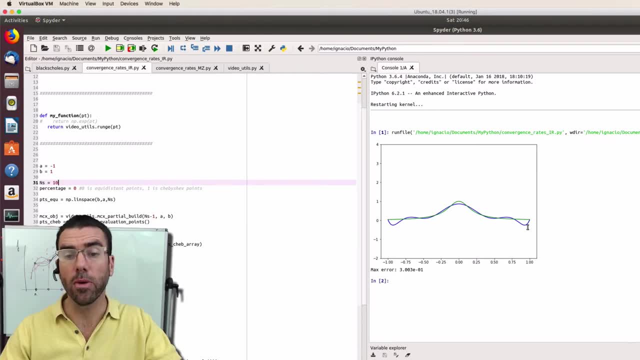 with, in this case, 10 points. So the polynomial of the green nine that goes through equidistant points, And here at the bottom underneath the graph you can see the maximum error of the approximation right Now. so we start with 10 points and we say, okay, this is what we get. 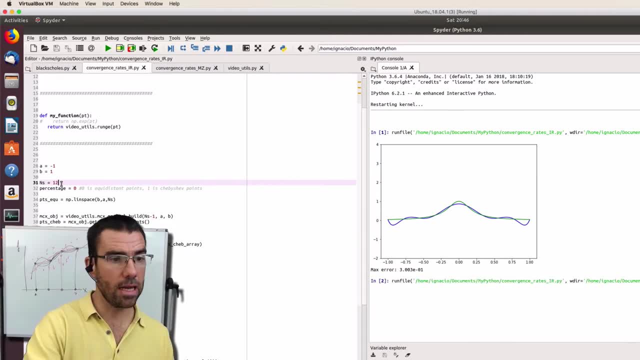 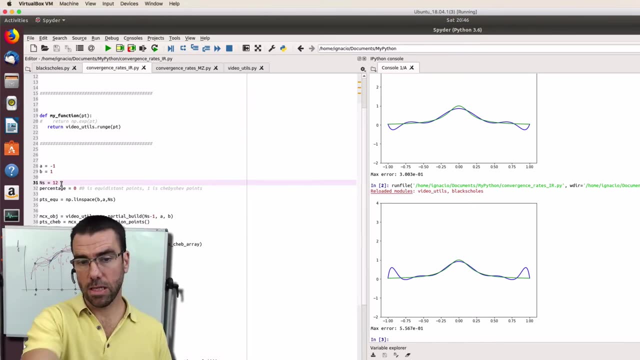 Now let's go, for example, to 12 points and let's run it again. You can see that it gets worse. Right, The error is bigger and you can see it in the graph. And just so you can see the number that I'm plotting there, that I'm showing there. Now let's get, instead of 12, 14 points. 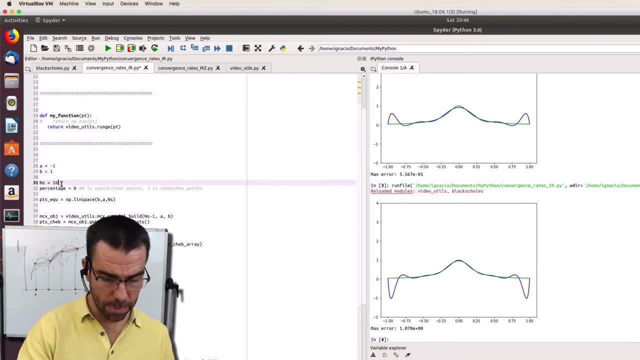 Again, it's getting worse. Let's get 16 points. It keeps on getting worse: 20.. It's getting worse and worse. Let's go to 25.. It's getting even worse. I mean this is quite a counterintuitive, because what we are doing here is we're saying that 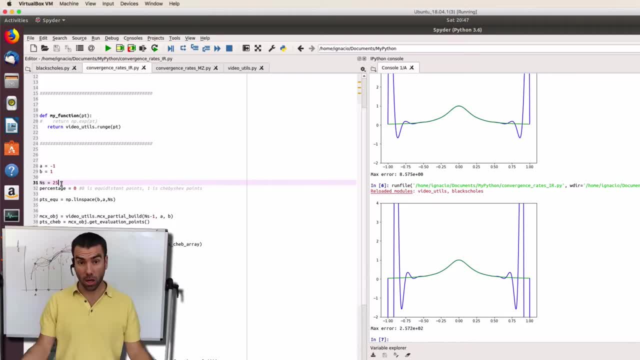 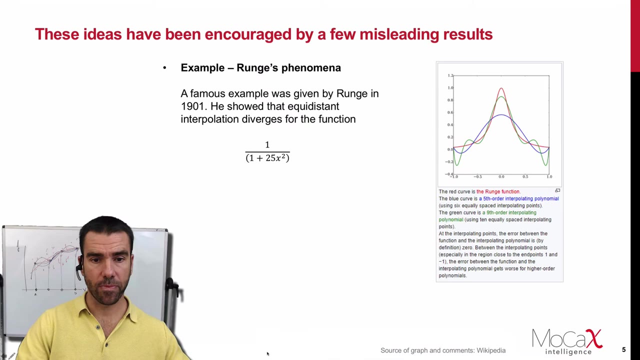 we're giving more information to the approximator And, in spite of that, the error is getting bigger. So this is quite a challenge, as you can see. Let me go back to the slides. Where am I Here? No, So this is quite a challenge And, of course, this type of results. 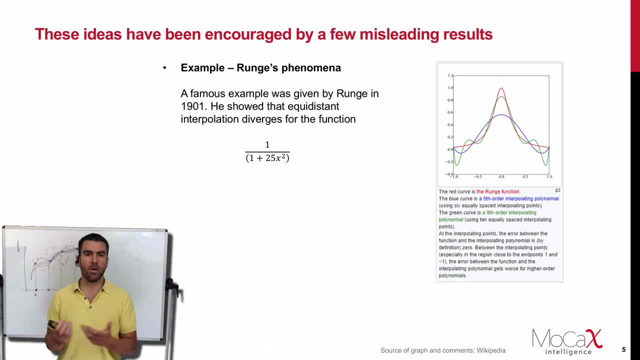 can be very frequently confused, even though we just have to remember that the result we're getting is now a couple of these two equations. So, for instance, we can see that when we take and we compute the byval, the function does the interpolation, But there is also just 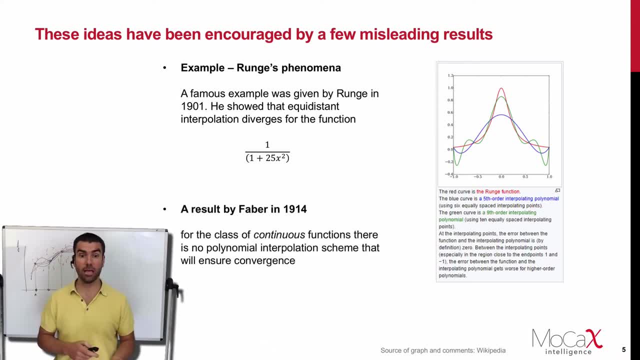 a slight delay. So we're just So, we're just. Well, to be fair, sometimes we see that. We see that if we just do a simple and smooth, a simple function, this function is analytical, It diverges, So the interpolation diverges. So let's not waste the time anymore with this. And in fact this was even more encouraged by the results by Faber in 1914, which he showed that for the class of continuous functions there is no polynomial interpolation in the scheme that will ensure convergence. So we have to interpret the function in a different fashion. 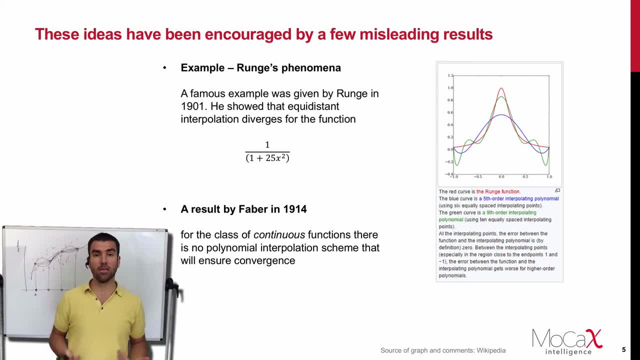 So you know, quite frankly, if you are told these things, you say, okay, let's forget about polynomials for approximation, They are a waste of time. That's what I would think in the face of this. All right, 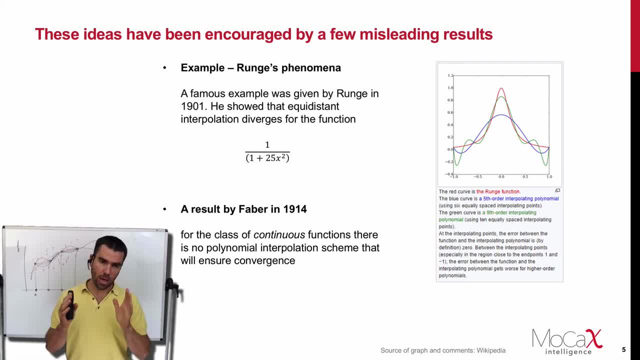 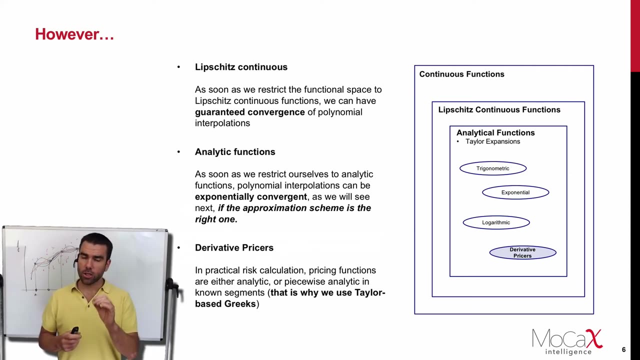 Fortunately, when we think along these lines, we have missed something. and we have missed something And I'm going to- this is what I'm going to show to you in this session- what we have missed, how to fix this. So what happens is that, as soon as we restrict ourselves to Lipschitz- continuous function- and, just as a reminder, Lipschitz continuity is just a very weak condition of continuity. 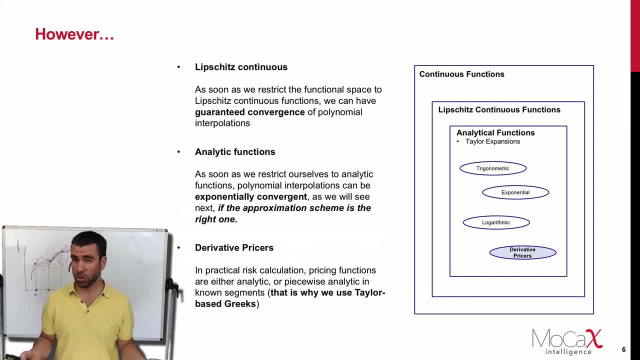 So basically, all real- or most the last majority of real life- functions are Lipschitz continuous. As soon as we restrict ourselves to Lipschitz continuous, we have guaranteed convergence. That's good On top of it. If we restrict ourselves to analytical functions, we not only have guaranteed convergence, but if we choose the right interpolation framework, we know we can demonstrate that it is going to be exponentially convergent. 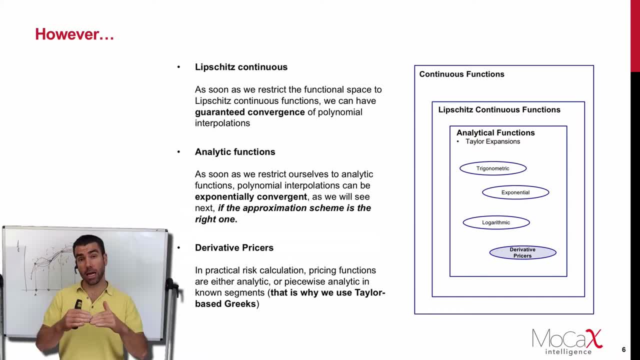 This is great. This means that we have a framework that we can, that if the function is analytical, we can approximate the function exponentially, And what that means in practice is that, with very few points, we can nail the function With a very high accuracy. 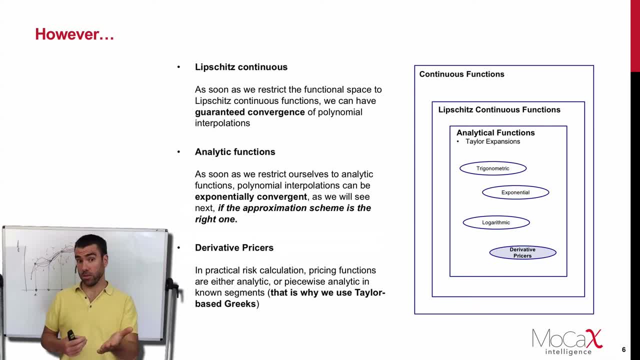 Now the derivative prices are actually analytical functions, And of course they are, because we use Greeks all the time to measure risk, right, And if you remember an analytical price, analytical function is one of the definitions. It's a function whose Taylor expansion converges in every point. 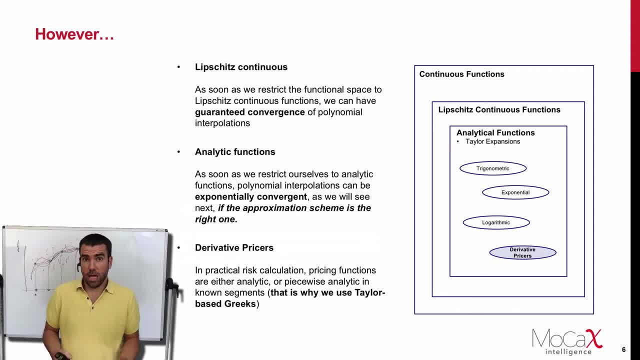 So when we use Greeks, which is the first or the second derivative, what we're saying is that, implicitly, we're saying that the price is an analytical function. So In the very, very worst case, a price there is analytical, piecewise, analytical by, in different, by blocks, right. 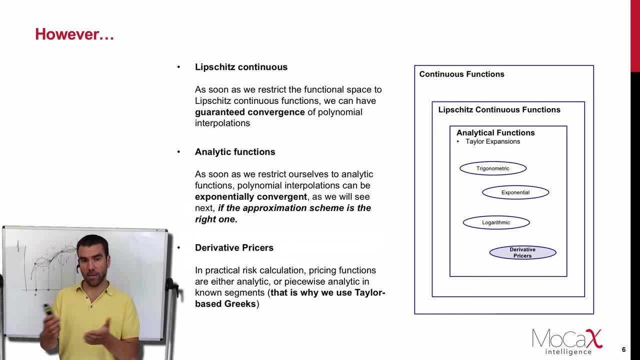 So, given that we have this framework, prices are analytical or, in the worst case, piecewise analytical functions, And we have a framework that we're going to see that is exponential convergence, Let's use it So, and this framework is the Chebyshev framework. 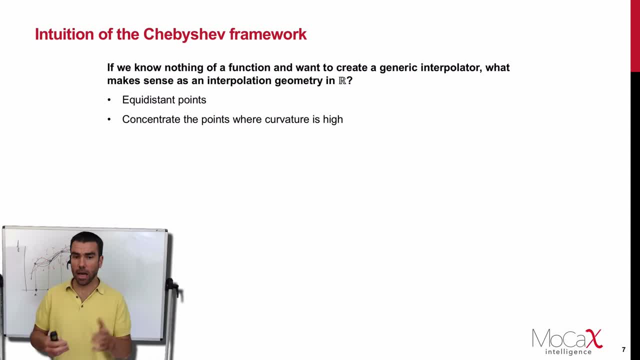 Let's get some intuition into how it works, As I have. As we have seen here, If we have a function and we know nothing about the function, what is my best guess as to if I want to approximate it with a number of points n. what is my best guess for where to put those points? 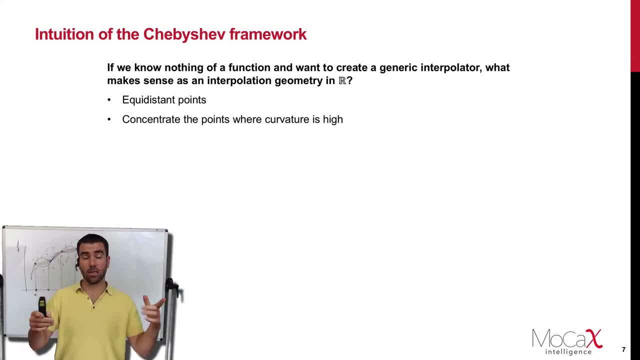 Well, the first thing to do is put them equidistant, right. That's what makes more sense. If we know something about the function, you can say: OK, what we can do is we can concentrate them around the curvatures, or what I mean by this is where the curvature is strong, or do these type of things. 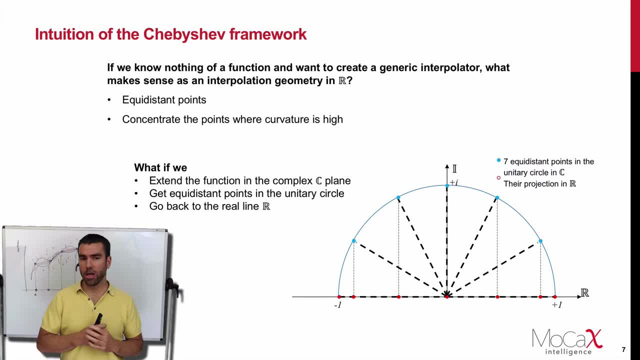 OK, that makes sense. However, what happens if we extend the function in a complex plane and then we get equidistant points in the unitary circle, as you can see in the screen, and then we project them to the real line, as you can see in the screen, and then so that we get to the red dots that you see in the plot in the screen? 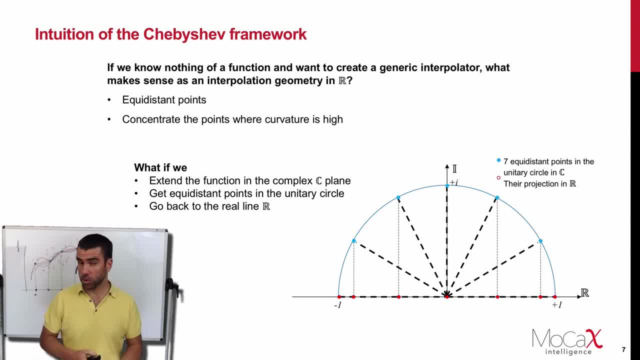 Those dots, the red dots, are the Chebyshev points, the so-called Chebyshev points, And it so happens that when we interpolate in the correct way, using that and using the Chebyshev spectra decomposition framework, we are going to achieve exponential convergence. 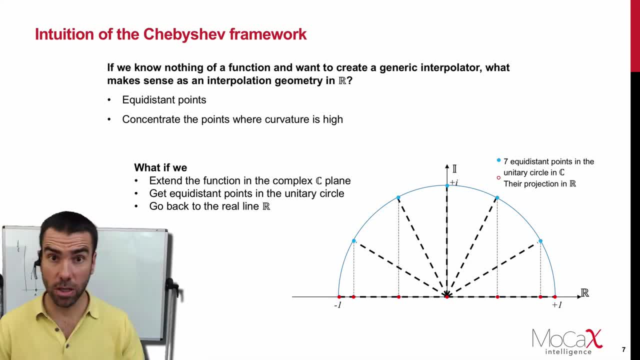 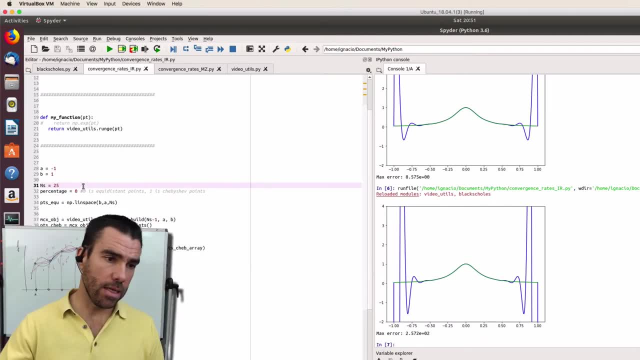 Let me show it to you. with the function that we were discussing before, the Runcke function, We go again to the Python And now I have this: Let me get my glasses so I know what I'm seeing. Let's This variable here: percentage in the code controls these points here: 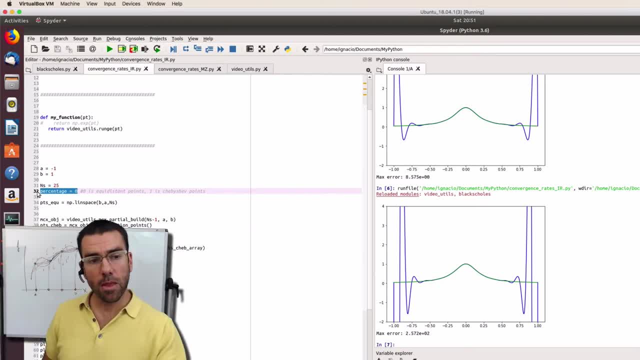 When this value is zero, I'm getting equidistant points. When this value is one I'm getting, we are getting Chebyshev points And the percentage what that does is it moves them. So if, for example, for four points, the Chebyshev points tend to, let me get this color. for example, Chebyshev points are going to be this one, this one. 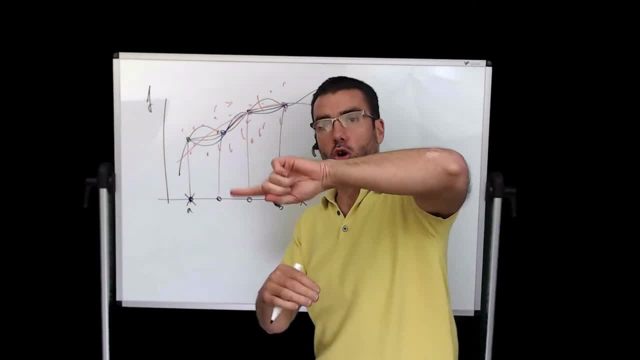 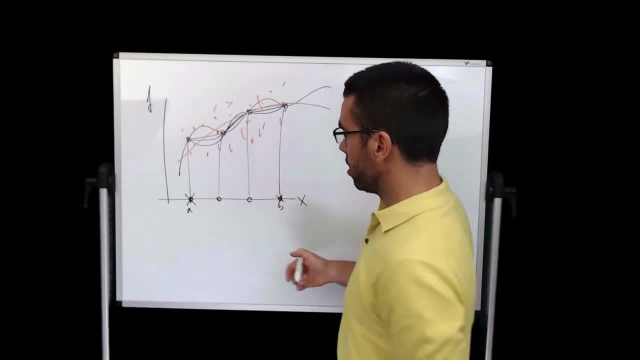 And then don't forget that, given that they are the projection of equidistant points in the unitary circle, in the complex plane, they tend to concentrate in the extremes. So the first four Chebyshev points are going to be this, this two and then this and this, approximately right. 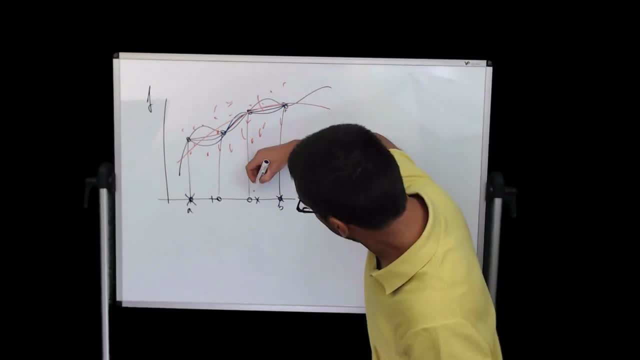 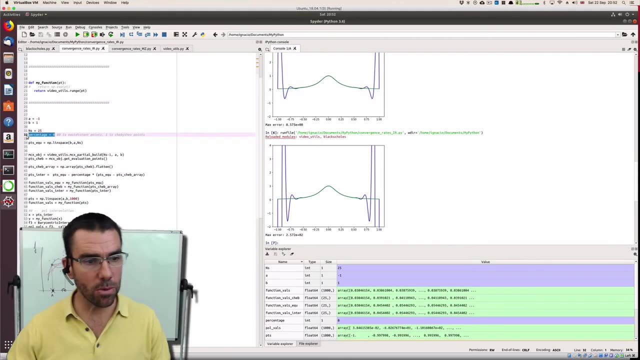 So this percentage variable in the code, what it's going to do is going to move this point from here to here and from here to that. Okay, So let's see what happens when we move it. We start at zero, which is what we had. 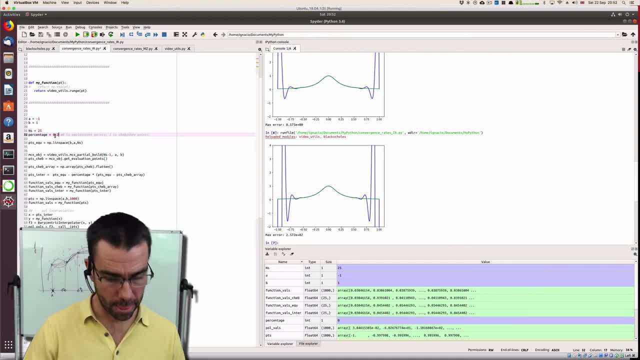 Now let's put it on 0.2.. Let's run this. Okay, It's getting better. Have a look at the error In the graph. it's more difficult to see, but we're going from 10 to the 2 to 10 to the 1 in error. 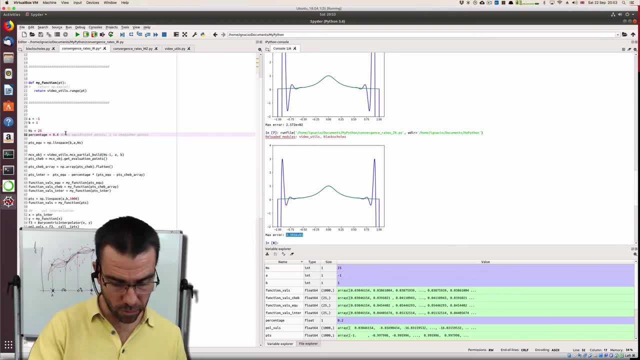 Ooh interesting. Now let's get to 40% closer. We is getting even better. The error is going to go to 4.. The other, The other, The other of magnitude of 10 to the other, of magnitude of 10 to the 0, or the 3.8 in this case. 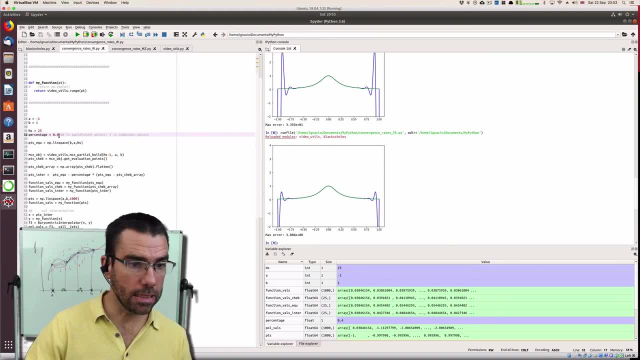 And you can see in the graph it's getting better. Now let's get it to 60%. Ooh, it's disappearing, the error. You can see it in the graph. You don't even need a number anymore. Now let's get to 80%. 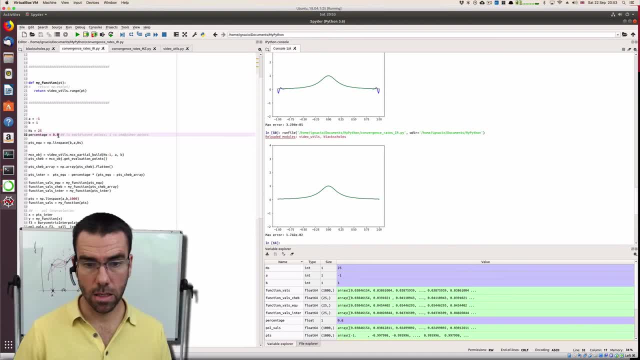 In the graph, it disappears, And now we have an error of 10 to the minus 2. Whereas in the one before it was 10 to the minus 1.. Let's get to the Chebyshev points One. 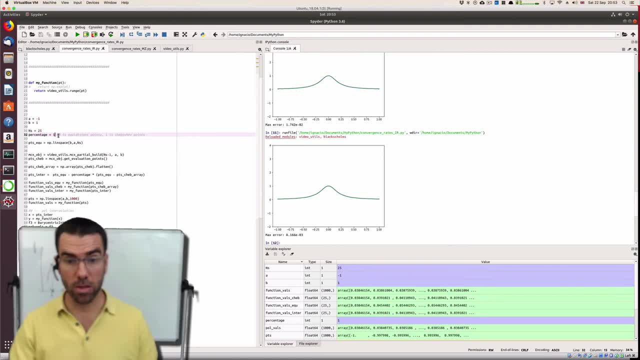 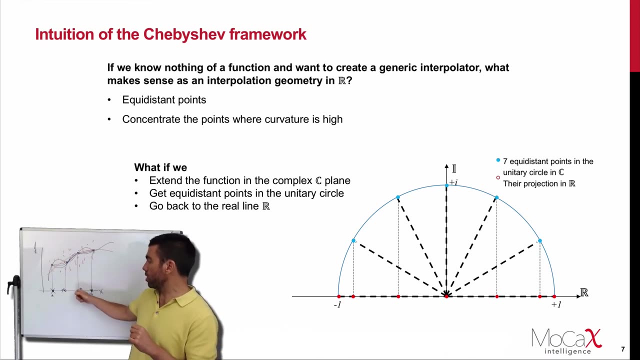 Look, we have an approximation error, maximum error of 10 to the minus 3.. The graph looks absolutely perfect. So you can see with this example, that by doing this- let me go back to the presentation- that by doing, by moving the points from the equidistant points to the Chebyshev points, 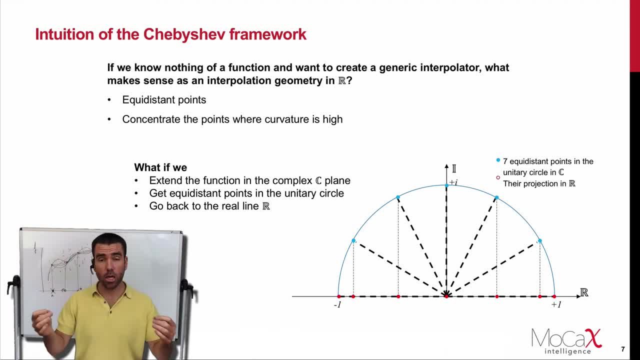 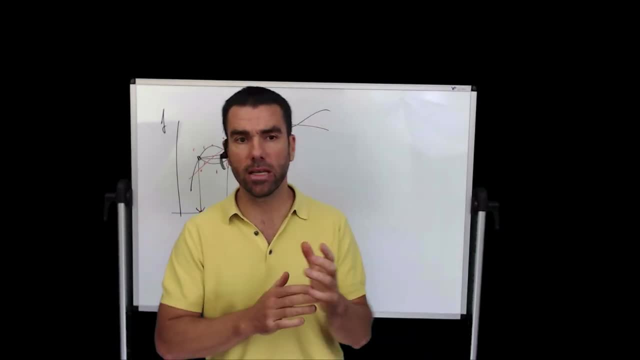 using the same, The same framework, which is an interpolant, we are reducing the error massively. okay, in fact, i was the other day, i was in a few months ago. i was in a in a forum, one of these online forums about the mathematics and and codes and and practicing of derivatives and this type of things, and they were talking. 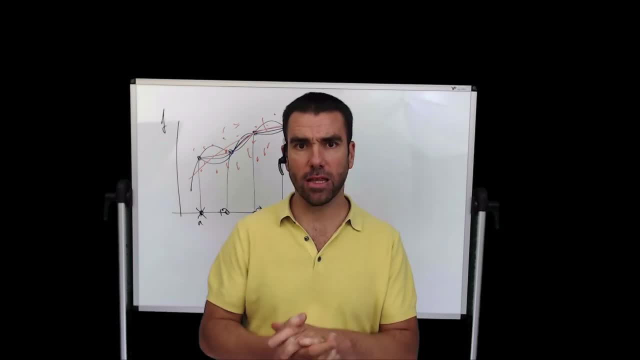 about the derivative points as the magic points, because they they seem to be magic. they seem to be like when you go to, when you use the derivative points to call your function and then you use that information in the correct way it is, you can approach the function in an amazing way, in fact.